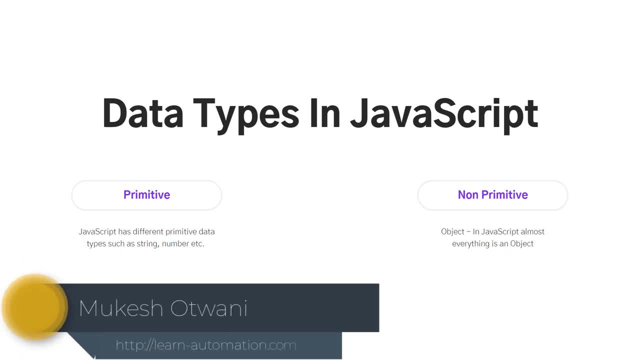 Hey everyone, this is Mukesh Yotwani, once again from learn-innovationcom. Today, in this lecture, we are going to talk about data type in JavaScript. As you know, data is the most important part for any programming language, right? 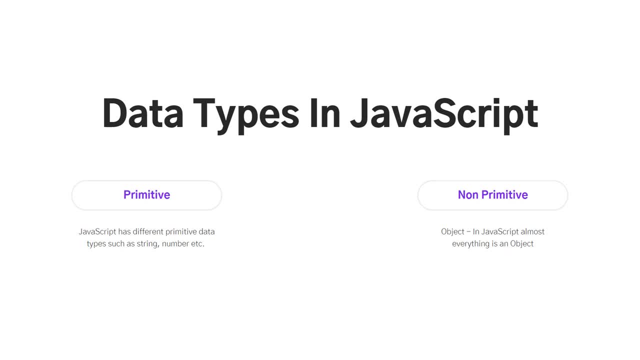 So once you understand how this data is getting stored, in which format is getting stored, then we can modify the data, we can do some operation right. So let's get started with data types in JavaScript. So basically, we have two categories here: One is primitive and second is non-primitive. 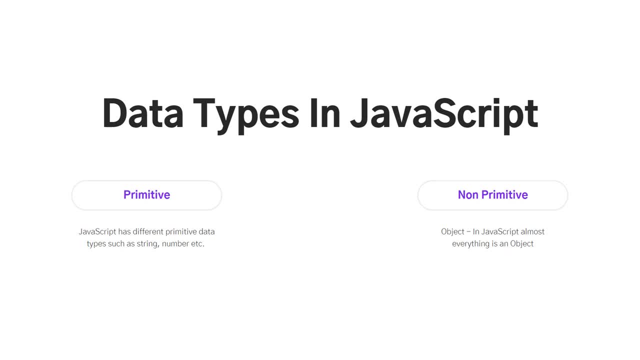 So, when it comes to primitive, we have different data types, which I will show you in the next slides, which are string, number, boolean, null, undefined, and so on. And the next category is non-primitive, or you can say reference data type. 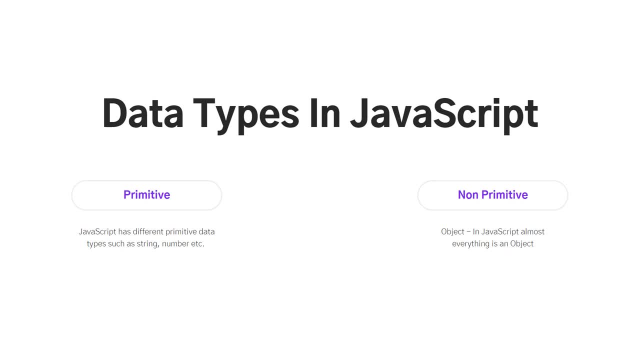 So good thing about JavaScript is almost everything in JavaScript is an object. okay. So once you move ahead, you will see everything which is not primitive is almost object here. Okay, so once you move ahead, we will have a dedicated session on non-primitive. This session is all about primitive, where we will be using 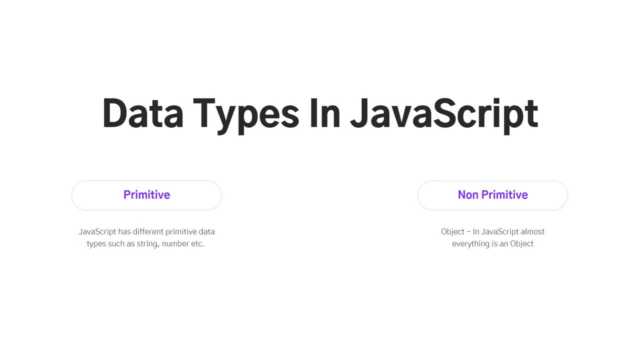 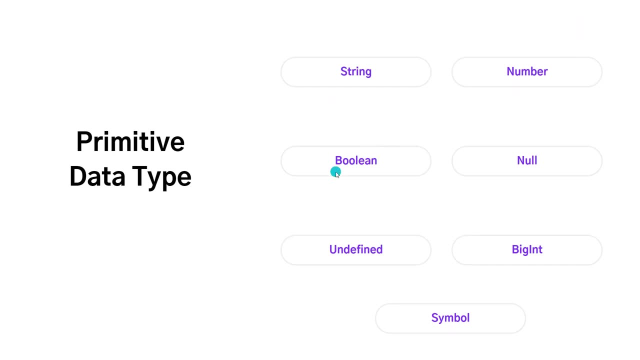 string, number, null, undefined and other primitive data types. Okay, so now, when it comes to primitive data type in JavaScript, we have string, we have numbers, we have boolean, we have null, we have undefined, we have big int Throughout the series. 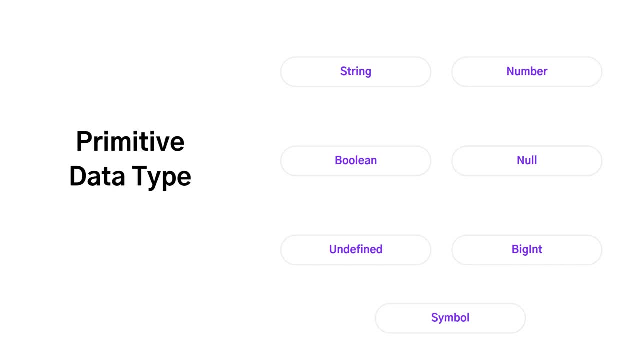 I will be talking about string, number, boolean, null, undefined, and we will not discuss big int and symbol in this course. But in case, if you're interested, please go ahead and you can check out these other two data types as well. 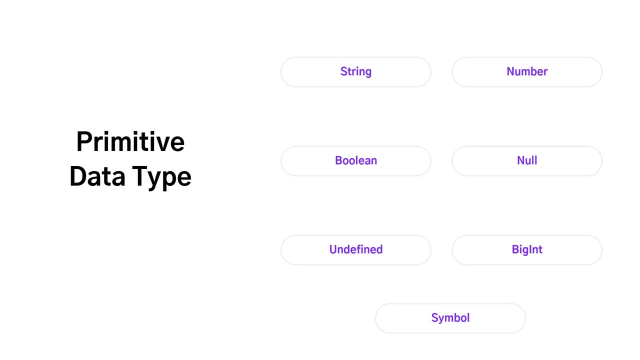 Okay, and before I move to the actual demo or the actual example, let me also highlight one point here: that, except null and undefined- all primitive data type that you are seeing on the screen- they have a wrapper object. okay, So once you move ahead, we will be. 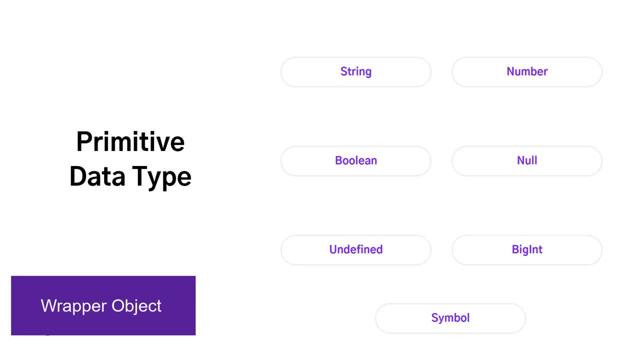 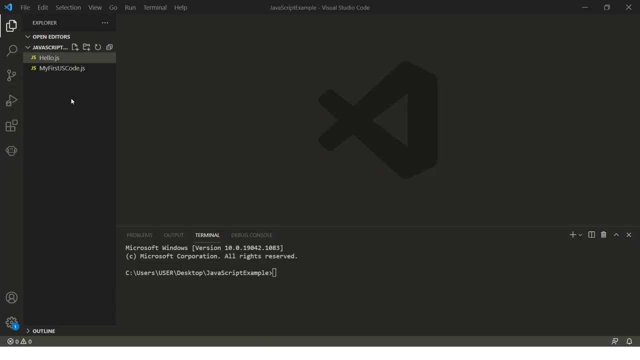 using this wrapper object terms very frequently. So just keep a note: except null and undefined, we have wrapper objects for each and every type. So let's create a new JavaScript file And let's understand all this data type. So I will create a new JavaScript file and 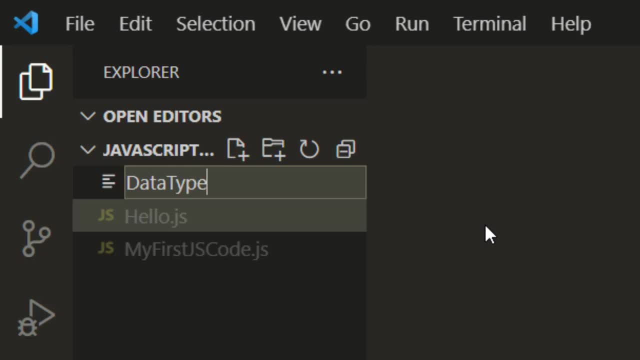 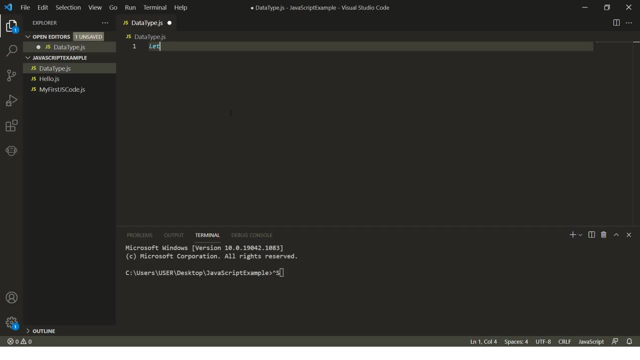 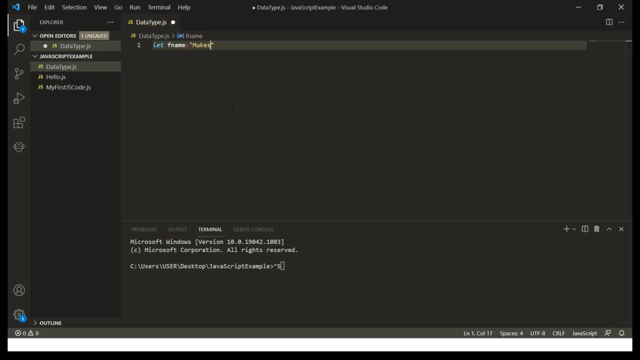 I will give this file name is data type demo or just a data typejs. So let's see how to get started. So I will be using let keyword. okay, And now let me just use one variable called fname, And I'm just giving my name in double quotes, which is: 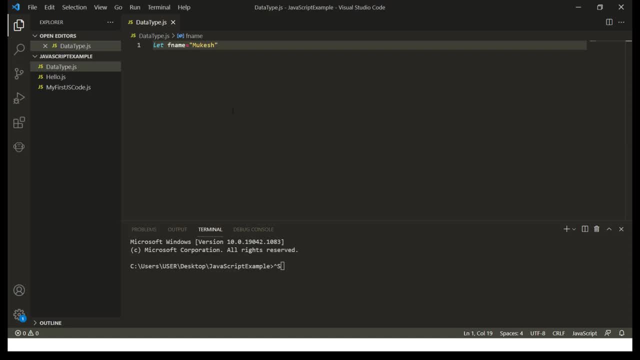 Mukesh. So this is fname, is a variable which is holding value as Mukesh. So if you just want to print, you can just say console dot, log And you can just give this name called fname. It should ideally print this value. So just write node and just give the file name. 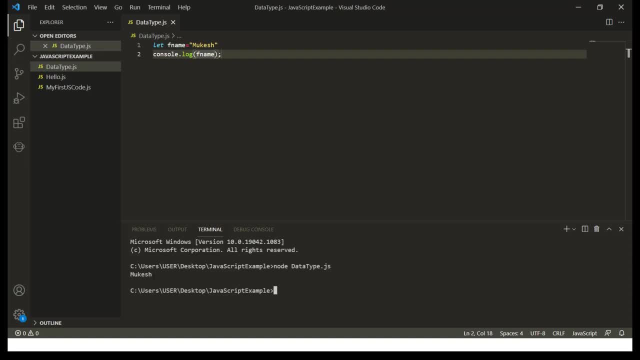 which is data typejs And you can see the value is Mukesh. But what is the type of this value? If you want to know in runtime you can just use something called type of operator. So if you just say console, dot log. 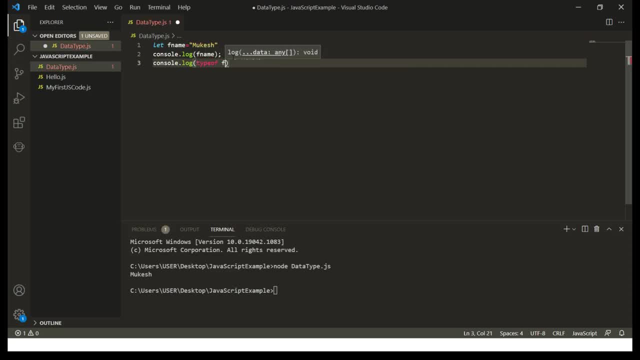 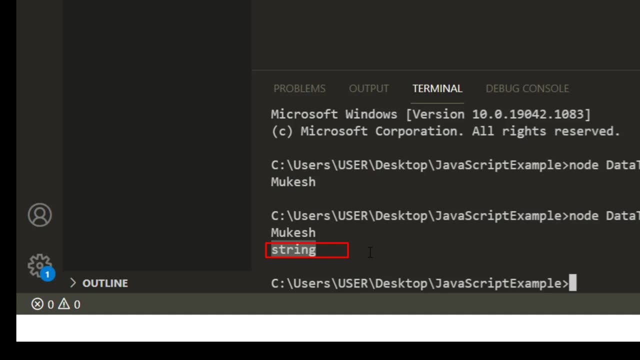 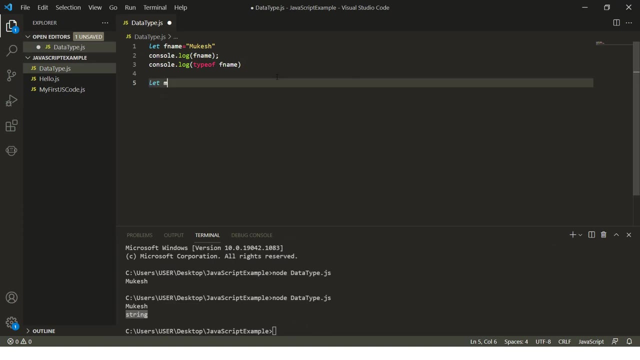 and now use this operator type of, and just type fname, So now it will also print the type of this variable. So, as you can see, it is giving us a string. So anything which is in double quotes, single quotes, it will consider as a string. In a similar way, let's say, if I just 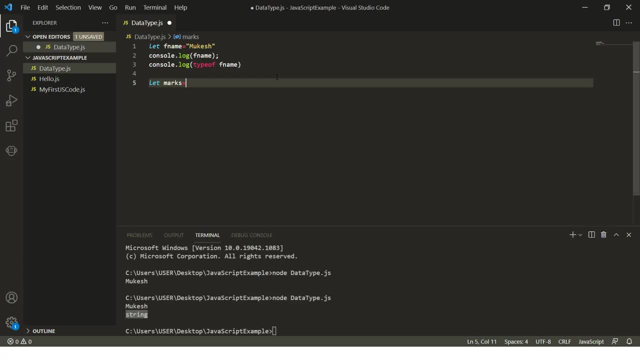 use one variable called marks. okay, and let me use, let's say, marks is 98.. Now if I want to print this, let's say I will use again console dot log. And if I say marks and let's also print the type of, so we can do one thing. let's print the first. 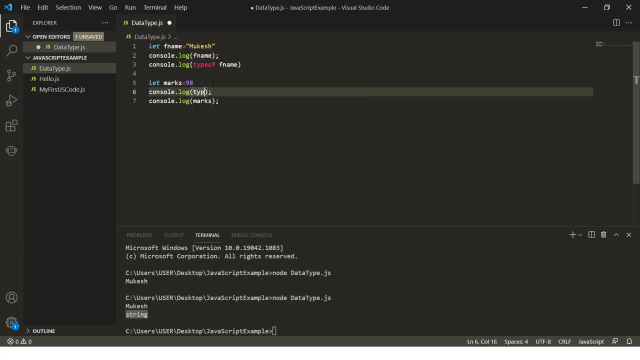 type of, then we will print the actual value. So I will say type of marks And let's see. So you can see: this is the number and marks is 98. So it's not only the integer value, you can have any floating value as well. So let's say, if I just gave 98.5,. 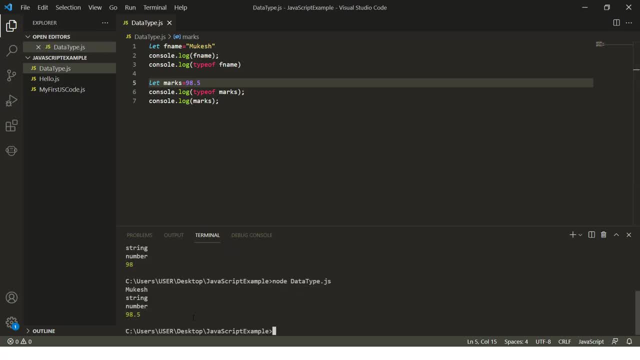 you can see, we'll still get the value as number, So you can give negative values as well. Okay, there's no issue. So if you are coming from different programming language like Java, where we have byte short in long flow, double here. 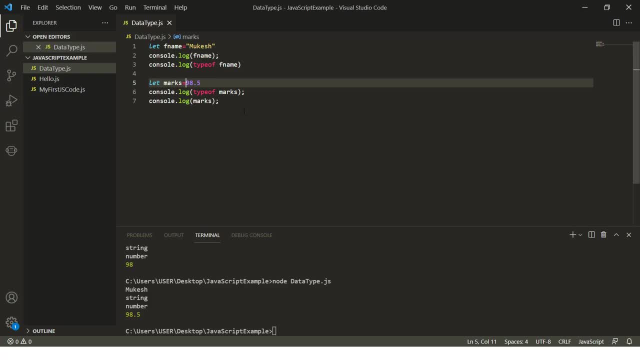 everything is a number. We also have begin, but that we will see in some other lecture. Now, if you talk about another type, we also have a data type called Boolean. Okay, so let's say, if I just use something called true, So now this status is a Boolean. 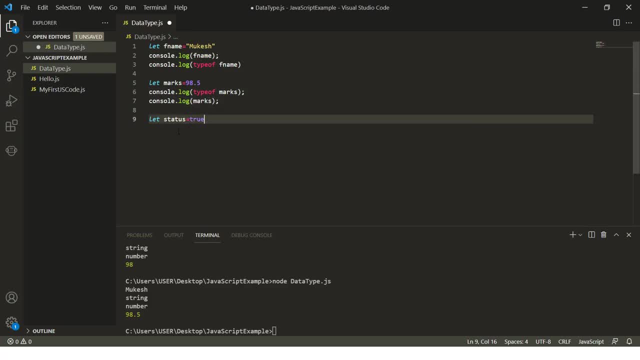 type. If you just want to know, just copy this And let's print. So I will say: type of status. I want to know the type of the status variable, so which will return you Boolean. And finally, I want to print something called status, which should give me the: 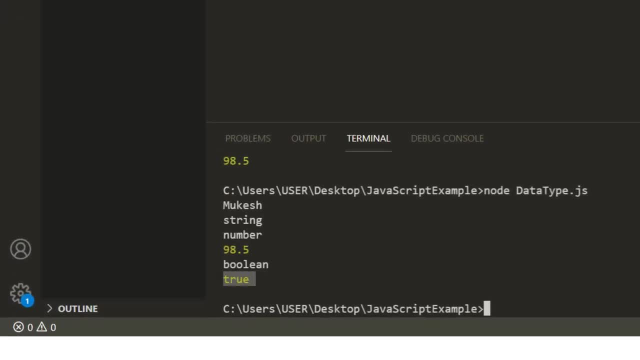 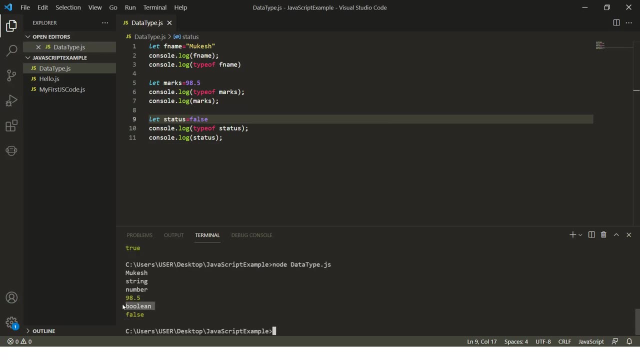 value. So, as you can see, it's a Boolean And the value is true. In a similar fashion, it can also hold false. And again, it's a Boolean Now in JavaScript, when you have some variables, okay, so 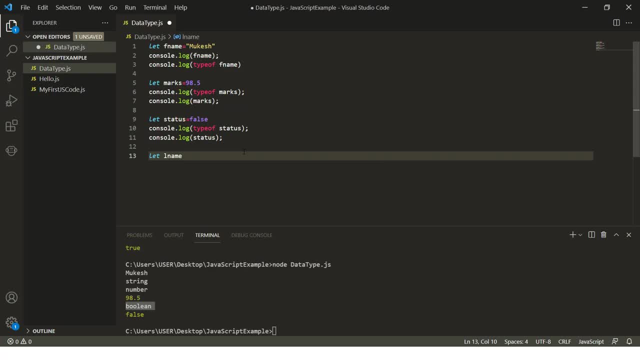 let's say, if I'm using one variable called lname, Okay, And now, the moment I will try to print this, I will say console dot log and I will just say lname. Let's see what it returns. The moment I run, you can see I will get something. 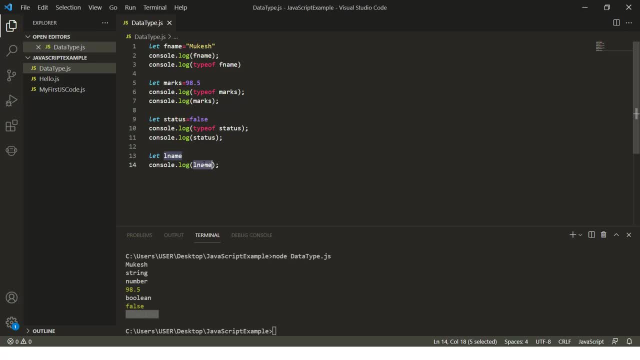 called undefined. We will not be getting null here. Null has a different use case. Whenever you have variable, when you don't have any value, it will give you undefined And if you want to see the type of- let's use it again- log just console dot. log, basically type. 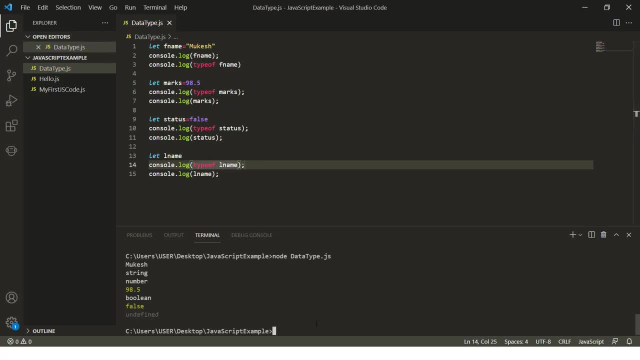 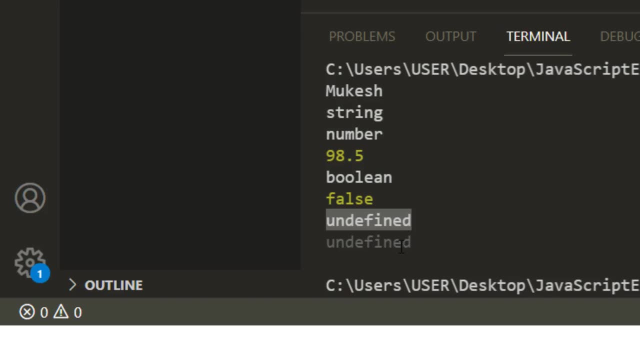 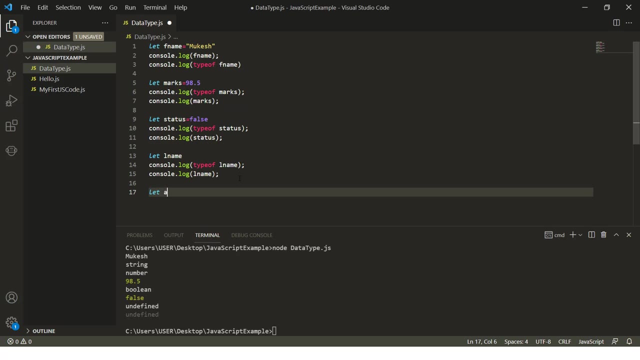 of lname, which is again undefined. So undefined is a data type and the value which is printing. basically it's undefined. Fine, And in a similar fashion, if I just use something called my address and if I just say null, now you will see a very interesting thing here: The 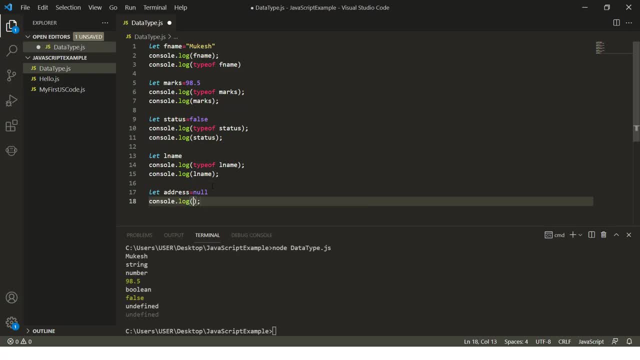 moment I say console dot log, obviously it will print null. Okay, as you can see. but the moment I use type of operator, you will see a weird behavior. Just type type of, just type address. So I just want to know the type of address. 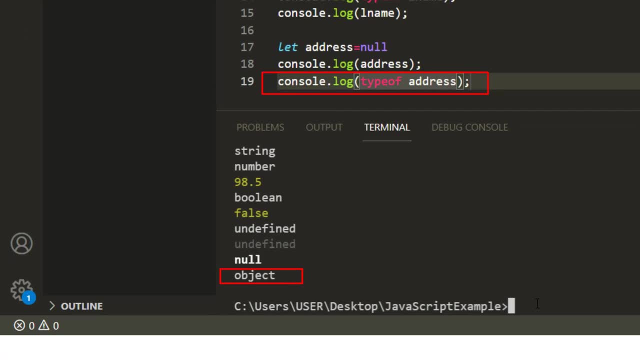 You will see something very different that it is giving you object. Okay, now I've gone through a couple of blogs, YouTube videos, a lot of posts, and I got to know there's a bug in JavaScript. even though it's a primitive data type, it will. 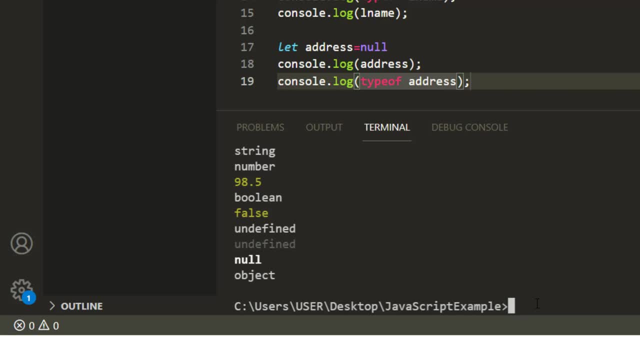 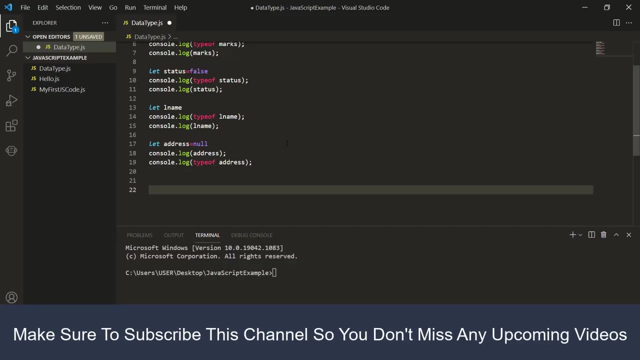 always present an object, which is sometimes confusing and frustrated for a lot of developers. But officially they have declared there was an initial bug in JavaScript. because of that, it is showing object, but it's a primitive data type, So keep this point in mind. So JavaScript is a dynamic typing. 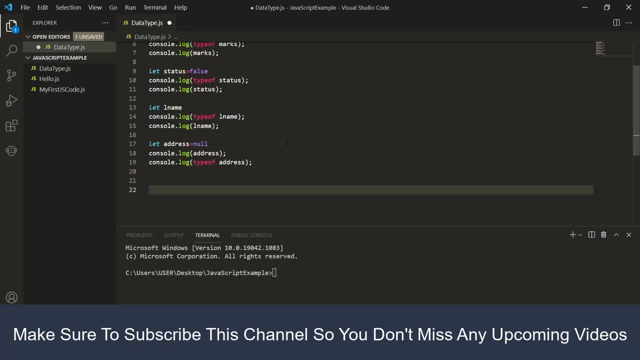 language What it means. when you declare a variable, you don't need to specify what type of variable it is Okay. so if you, coming from Java background, you must have seen we write: integer x equal to 10, double b equal to some value of boolean, c equal to. 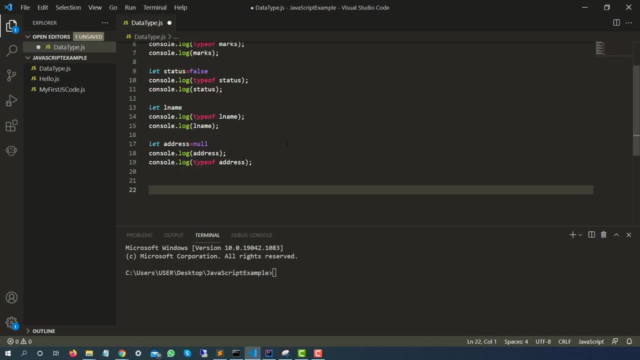 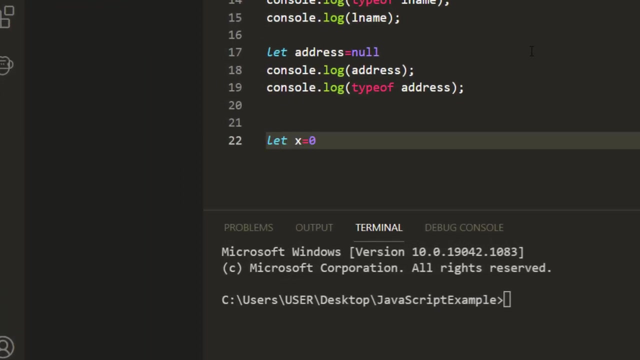 some value right where we define what kind of variable it is. But it's a dynamic type in language where you don't need to specify the data type. JavaScript engine automatically identify what kind of variable it is depends on what value you're assigning. For example, if I say let x equal to 10, it will. 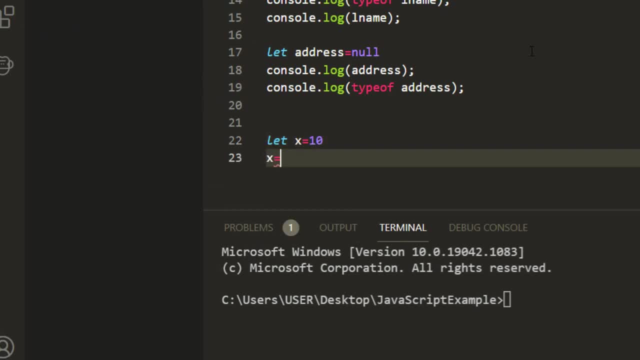 consider this as a number. But if I say x equal to true, it will consider this as a boolean. If I say x equal to Mukesh, it will consider as string. In a similar fashion, if I say x equal to- let's say- undefined, it will consider this as undefined. and 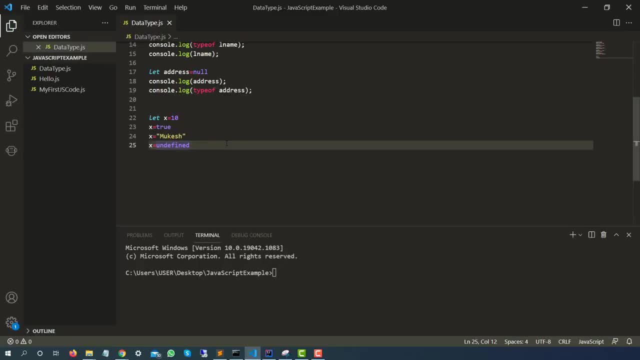 similar goes for null. Well, so let me quickly print these values. So what I will do, I will just say console, dot, log, And let me just print this x, And I will just print after every assignment: okay, And let me. 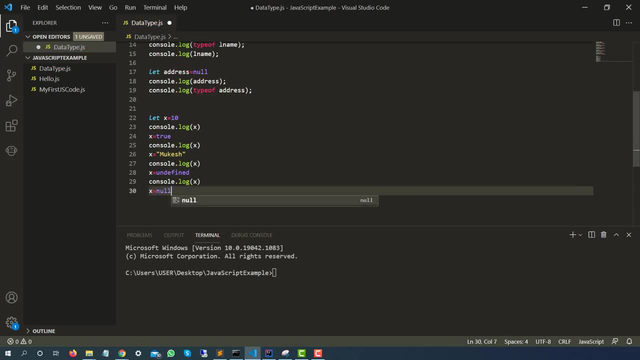 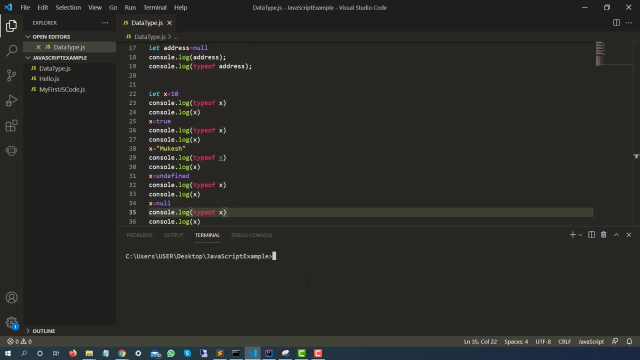 also assign x equal to null. And let me print this again: console dot log x. Let me just also write console dot log type of x. And I will just quickly add before printing: And same goes here. Now let's type node and let's give the file. 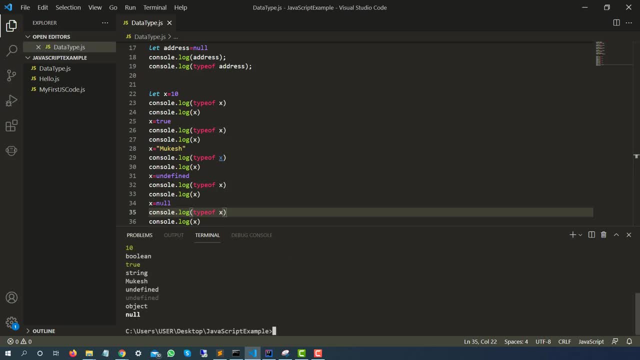 name, which is data type, dot j, s, And you can see initially, if we just scroll this up here: Yeah, number 10.. Then we are assigning x equal to true, So it became boolean, As you can see the value. then we assign Mukesh, So it will become it is. 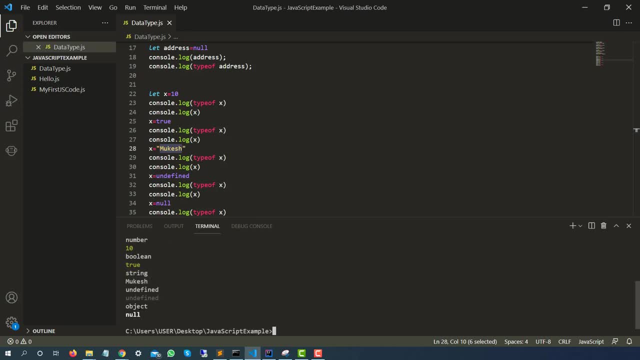 converting into string and values. Mukesh, in the same way, undefined And, as you have seen, for null it always give you object, So don't get confused with that. So these are the different data types we have. Now let me also show you one. 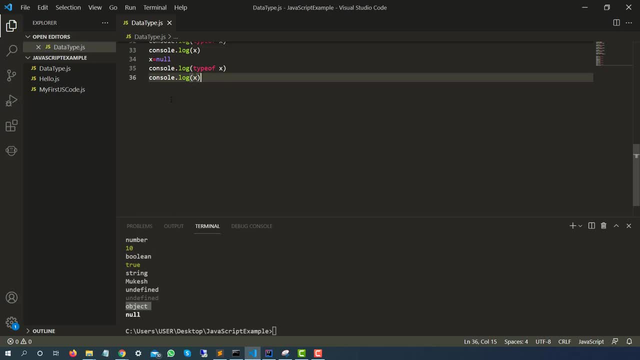 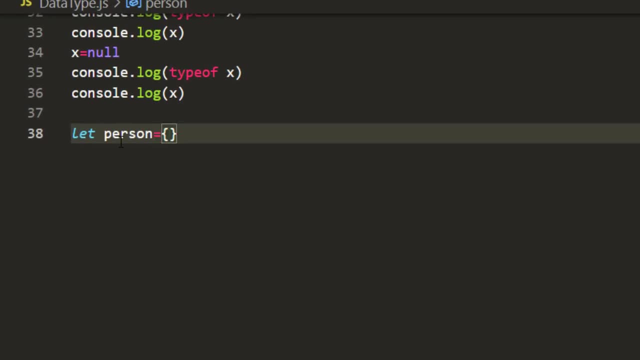 let's say I want to define one object here, Okay. so let's say I want to define one object here: Okay, so this object, I will say object here. Okay, so this object, I will say object here. Okay, so this object, I will say person object. And when it: 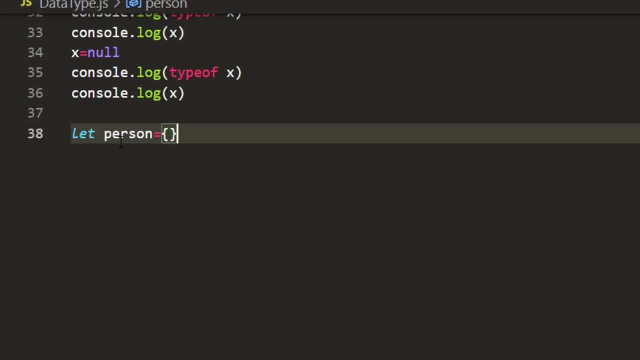 this object, I will say person object. And when it this object, I will say person object. And when it comes to object, you just person object. And when it comes to object, you just person object. And when it comes to object, you just need to write curly braces. 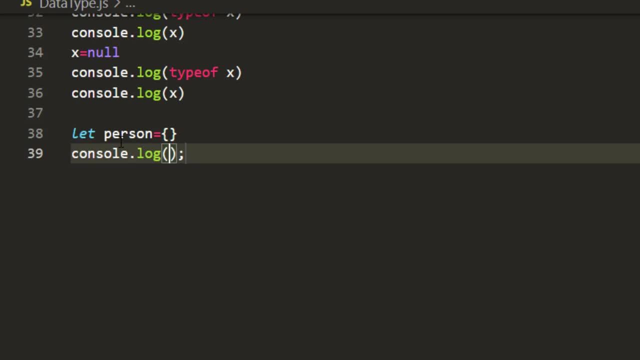 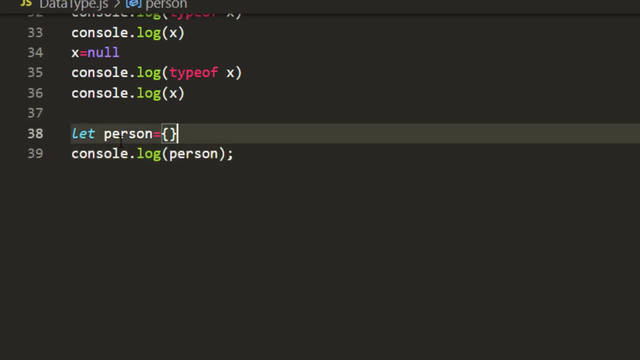 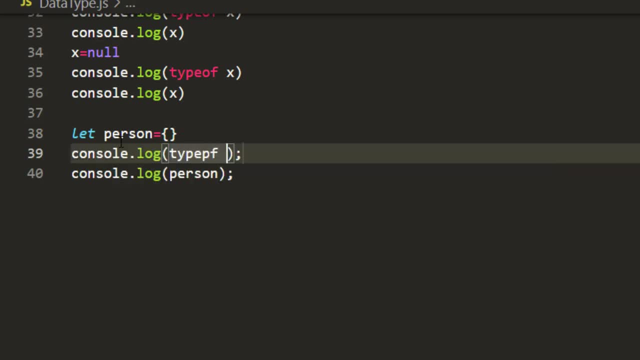 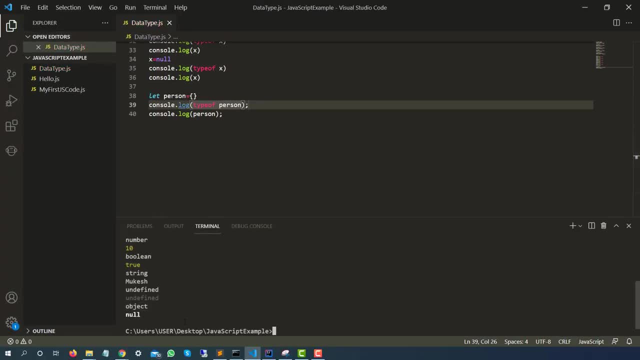 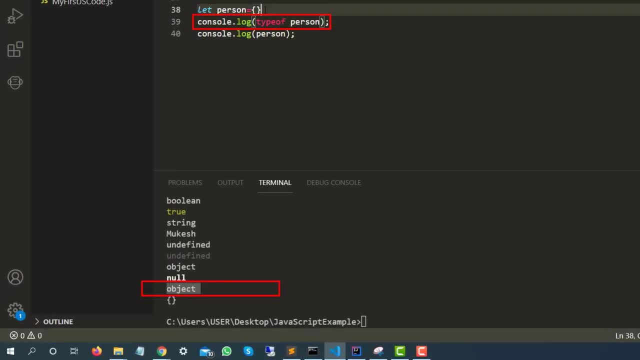 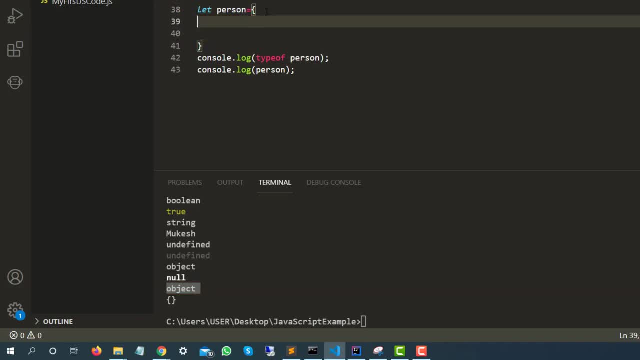 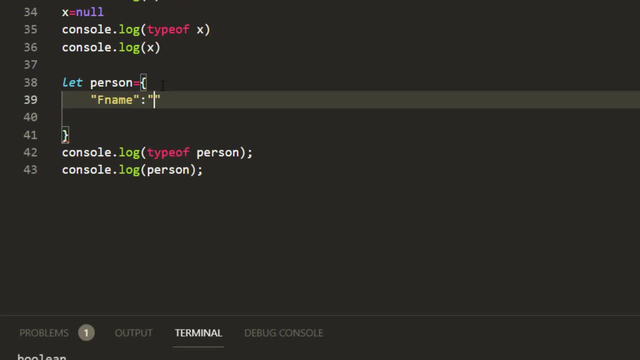 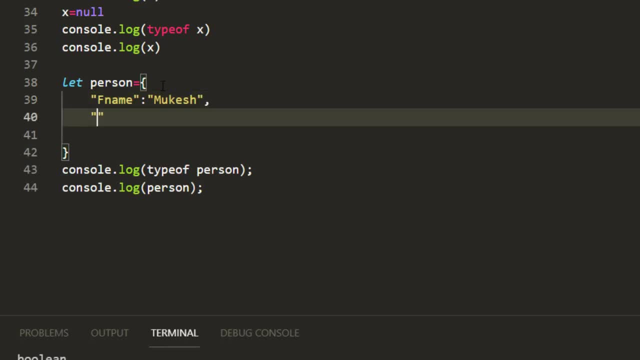 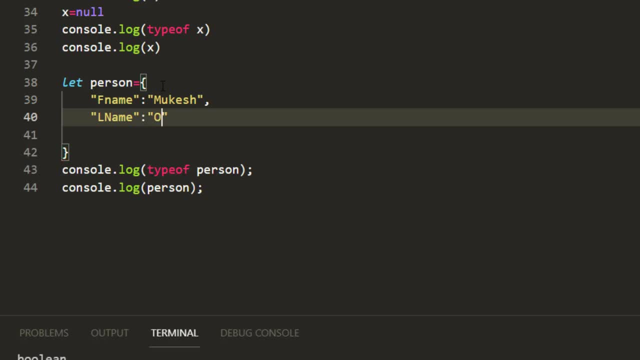 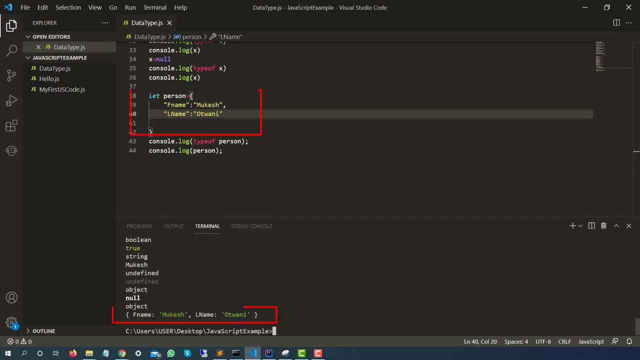 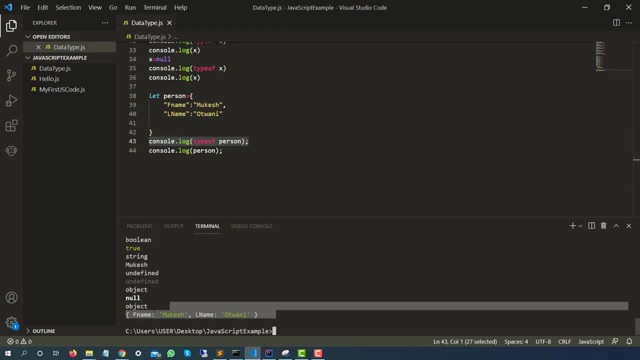 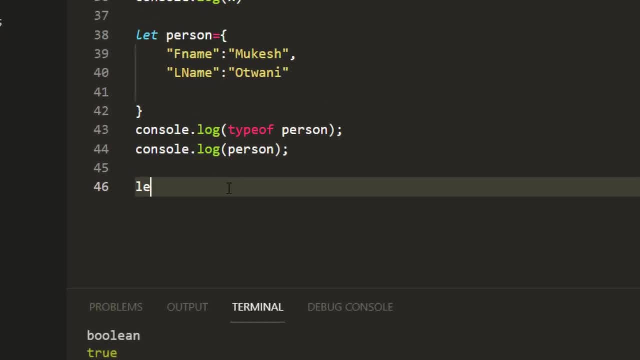 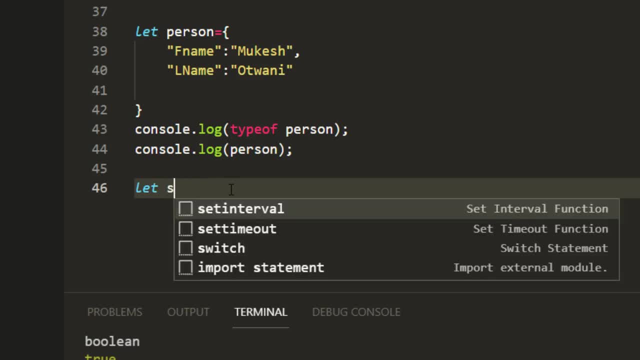 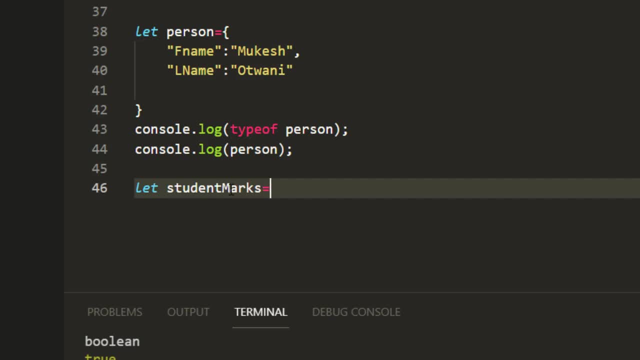 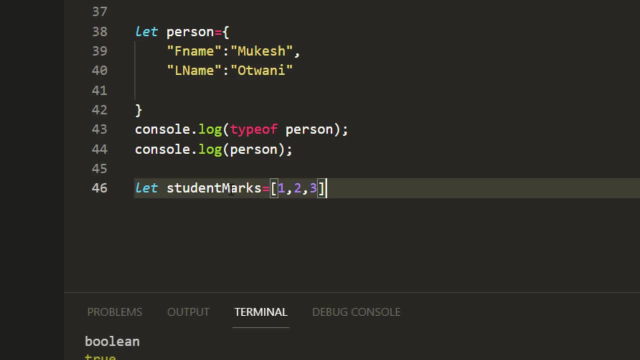 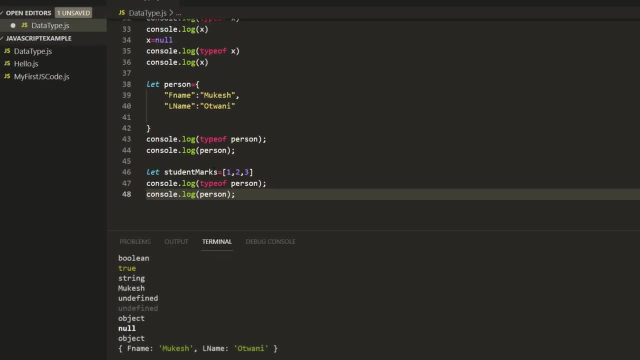 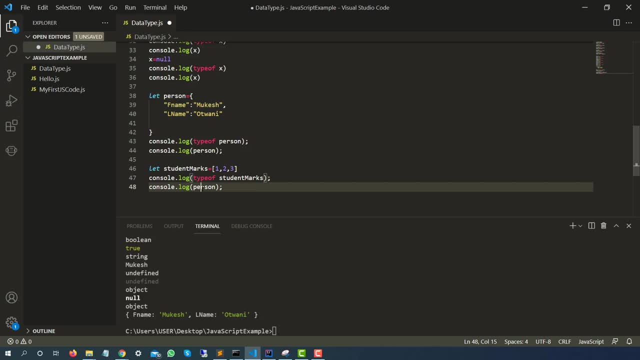 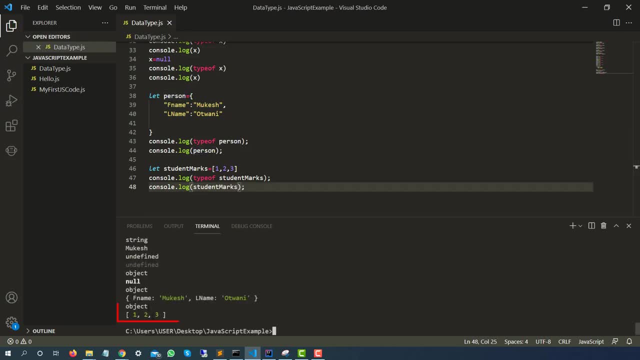 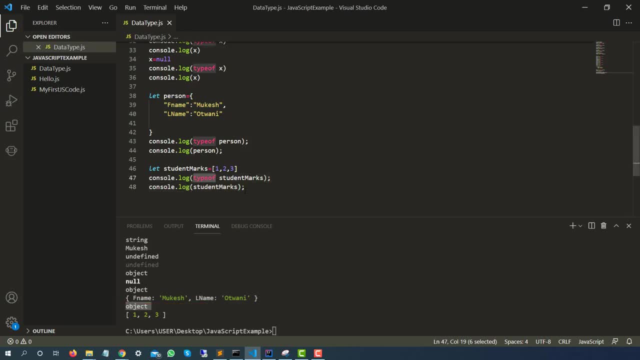 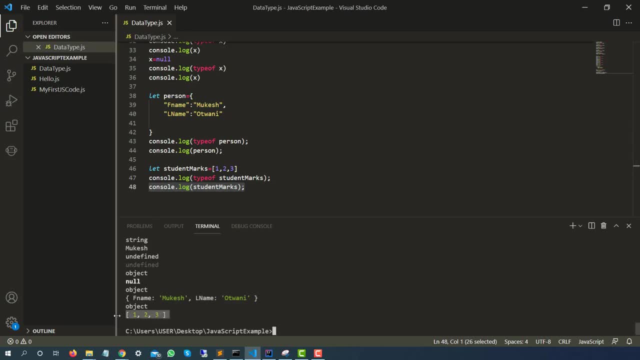 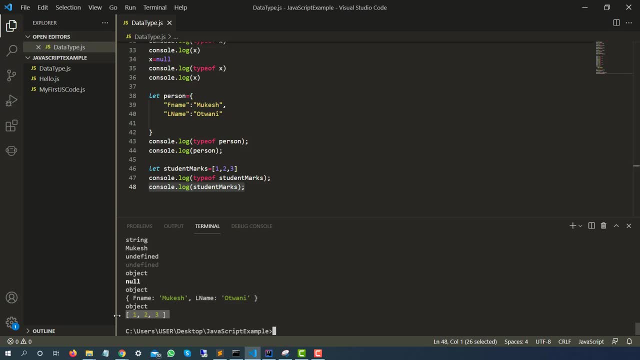 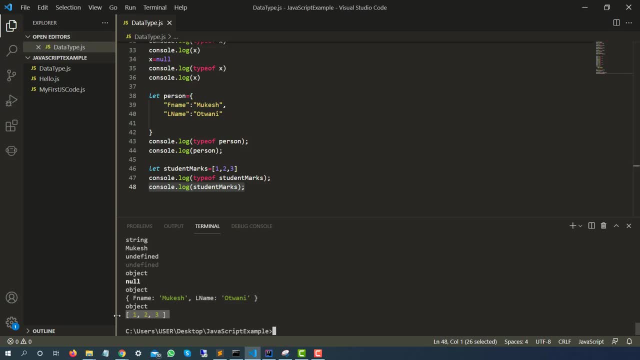 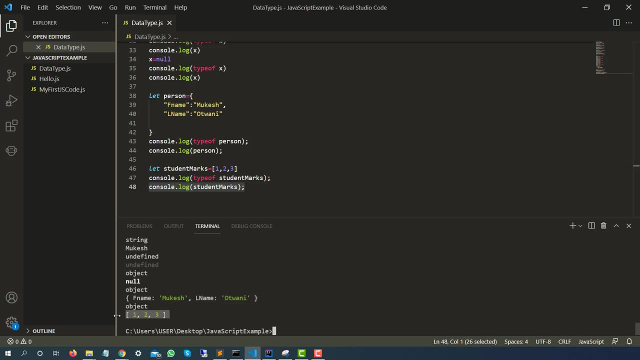 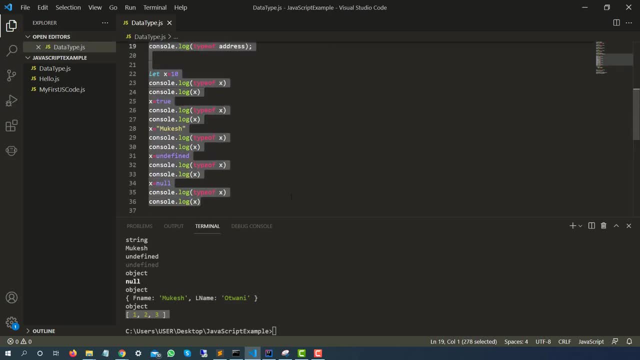 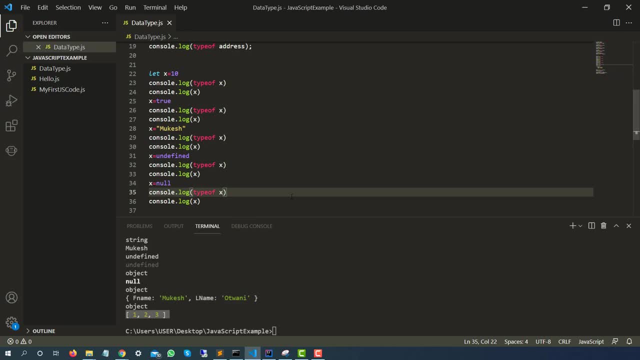 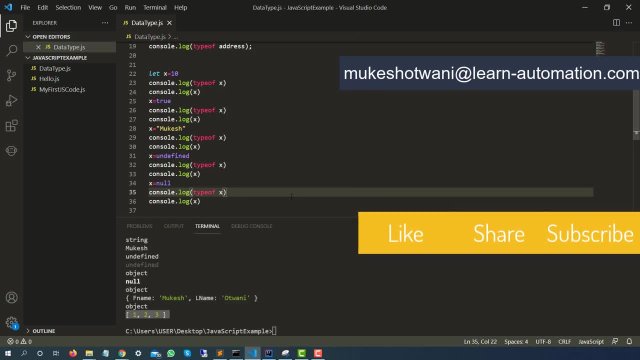